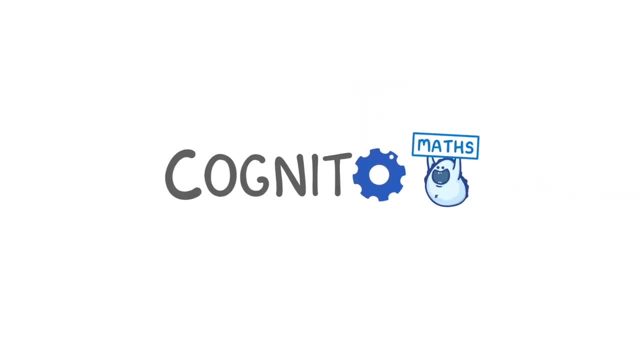 In this video we're going to see how to calculate the area of a sector and the length of an arc. To quickly recap what these terms mean, remember that when we take a slice of a circle like this, we get a minor sector contained within a minor arc and the two radii. 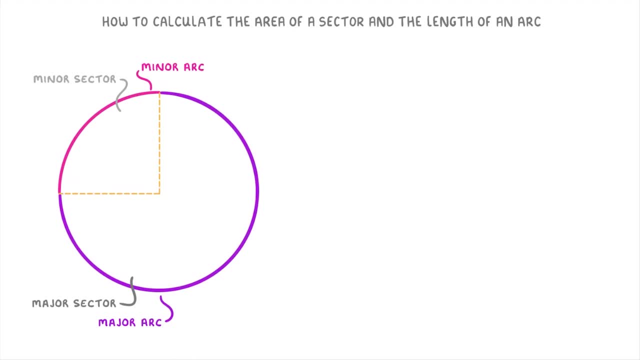 and a major sector contained within a major arc and the two radii, And when you get questions about this stuff in the exam, they're normally going to give you this angle here of the minor sector and the length of the radius. Now, if you want, you can just memorise these two. 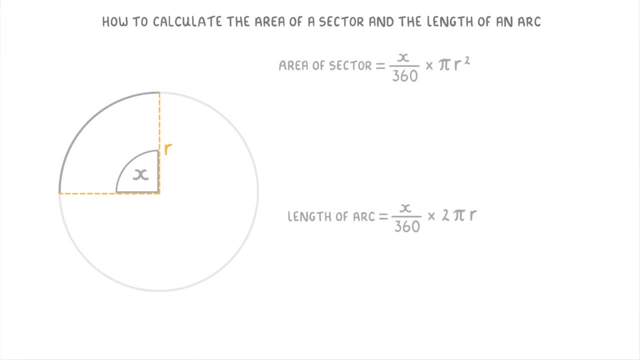 formulas here, and by plugging in the angle as x and the radius as r, this will give you the area of a sector or the length of the arc. What I want to do in this video, though, is go through the concept behind the formulas so that they make sense. 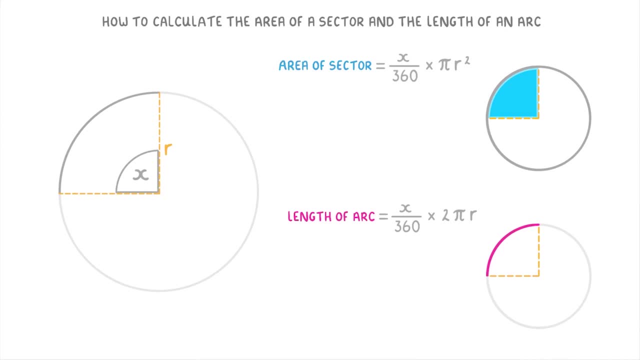 Because when we break them down they're much easier to understand and they're also a lot easier to use in tricky questions. So for me personally, the best way to think about this topic is to think about how big the sector or arc is as a fraction of the entire circle. For example, if our angle here 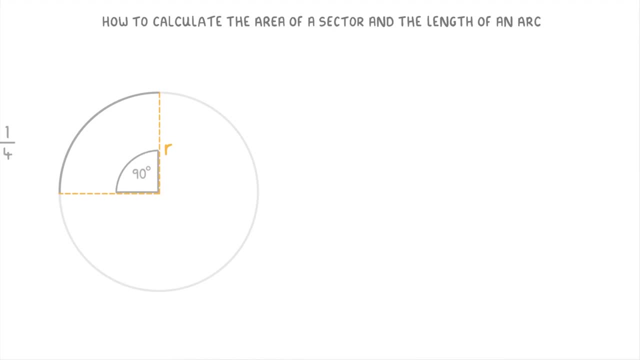 was 90 degrees, then that would mean that our sector was one-quarter of the full circle, Because, remember, a whole circle is 300 degrees, 360 degrees, and 90 is one quarter of 360. And so this means that the area of this sector would be 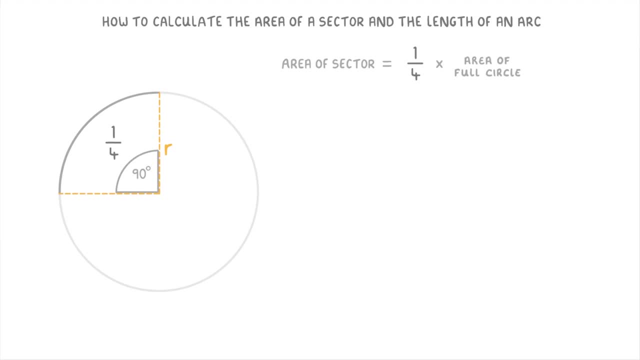 one quarter of the area of a full circle And the length of the arc would be one quarter times the circumference of the full circle. So to find out the area of our sector, we're going to just do one quarter times pi r squared, because pi r squared is the formula for the area of a circle. 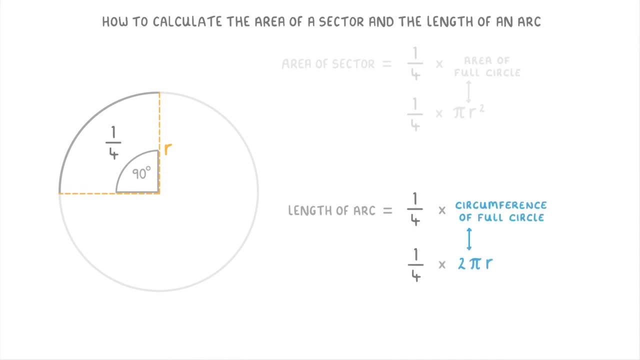 And then for the length of the arc we're to do one quarter times two pi r, because two pi r is the formula for the circumference. So if the radius of our circle in this case were six centimeters, for example, then the area would be one quarter times pi times six squared. 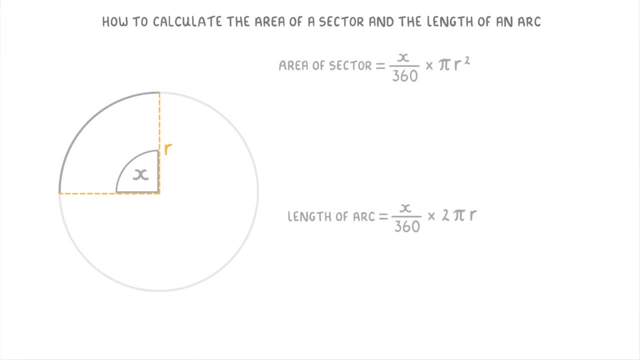 formulas here, and by plugging in the angle as x and the radius as r, this will give you the area of a sector or the length of the arc. What I want to do in this video, though, is go through the concept behind the formulas so that they make sense. 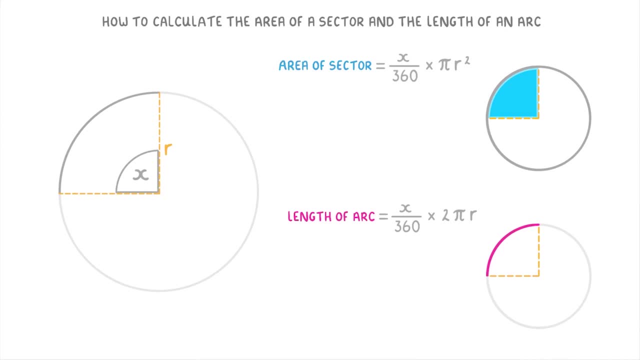 Because when we break them down they're much easier to understand and they're also a lot easier to use in tricky questions. So for me personally, the best way to think about this topic is to think about how big the sector or arc is as a fraction of the entire circle. For example, if our angle here 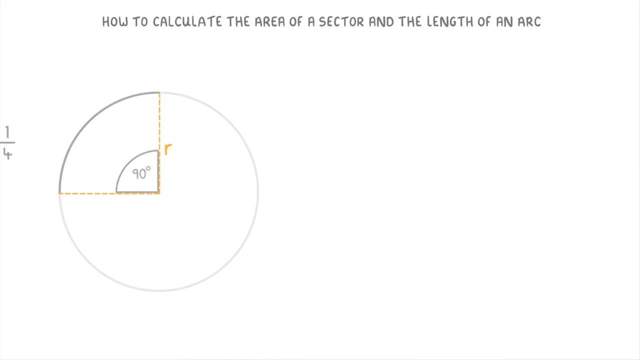 was 90 degrees, then that would mean that our sector was 1 quarter of the full circle, Because, remember, a whole circle is 300 degrees And 90 is 1 quarter of 360. And so this means that the area of this sector would be 1 quarter. 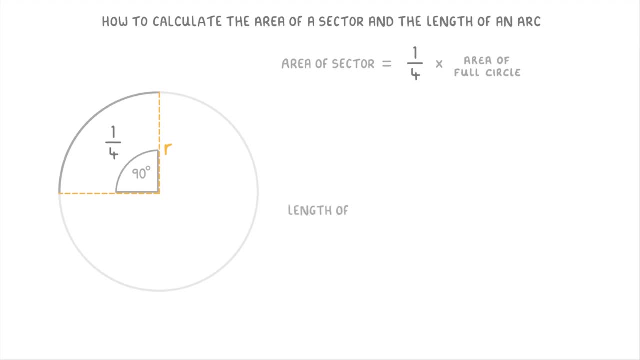 of the area of a full circle, And the length of the arc would be 1 quarter times the circumference of the full circle. So to find out the area of our sector, we'd just do 1 quarter times pi r squared, Because pi r squared is the formula for the area of a circle. 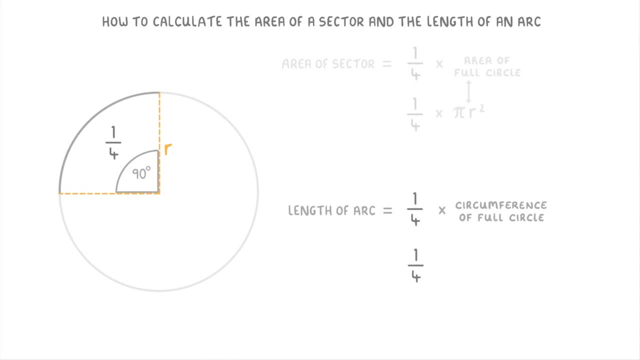 And then for the length of the arc we'd do 1 quarter times 2 pi r, Because 2 pi r is the formula for the circumference. So if the radius of our circle, in this case were 6 centimeters, then the area would be: 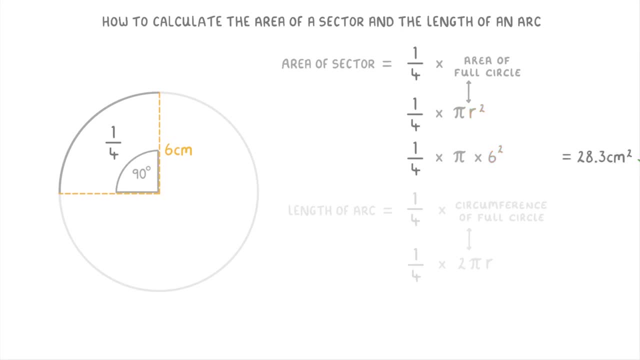 1 quarter times pi times 6 squared, which is 28.3 square centimeters, And the length of the arc would be 1 quarter times 2 times pi times 6.. Now this technique works just fine if you've got something easy like a quarter, a third. 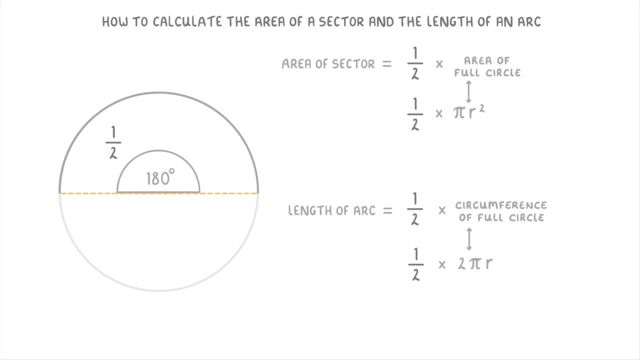 or one half of a circle. The issue, though, is that if you have a more complicated angle, like, say, 113 degrees, then it's a bit harder to know what fraction of a circle you have. In these cases, you need to write your fractions with a denominator of 360, because there are 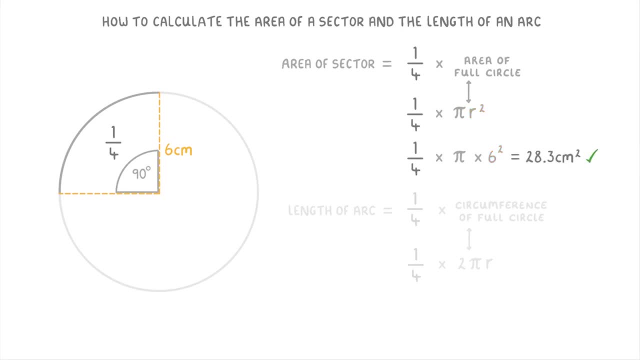 which is 28.3 square centimeters, And the length of the arc would be one quarter times two, times pi times six, which is 9.42 centimeters. Now this technique works just fine if you've got something easy like a quarter. 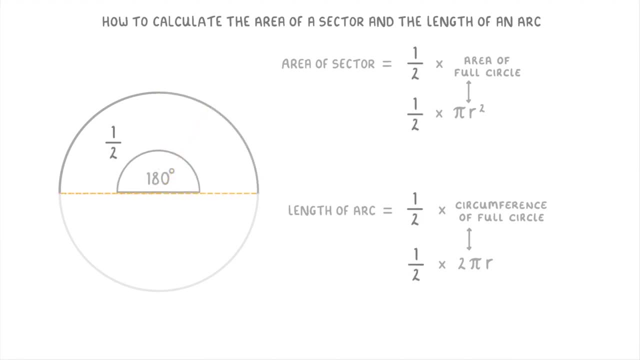 a third or one half of a circle. The issue, though, is that if you have a more complicated angle, like, say, 113 degrees, then it's a bit harder to know what fraction of a circle you're going to have. In these cases, you need to write your fractions with a denominator of 360,. 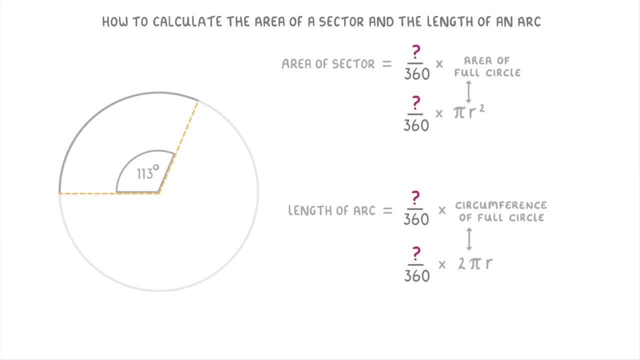 because there are 360 degrees in a circle in total, And then you just place whatever angle your sector is as the numerator. So in this case, because the angle of the sector is 113 degrees, our fraction would be 113 over 360.. Or in other words, our sector is 113 three hundred and sixtyths. 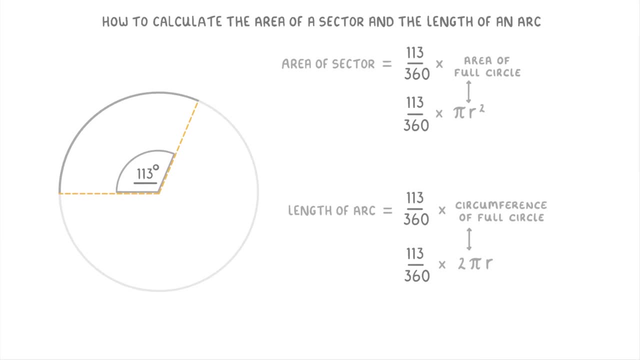 of the circle. So if the radius this time was 15 millimeters, then to find its area we'd do 113 over 360 times pi times 15 squared, which would be 222 square millimeters. And to find the length of the arc we'd do 113 over 360 times 2 times pi times 15, which is 29.6. 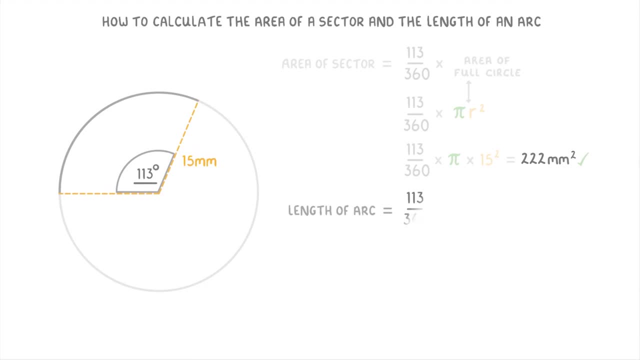 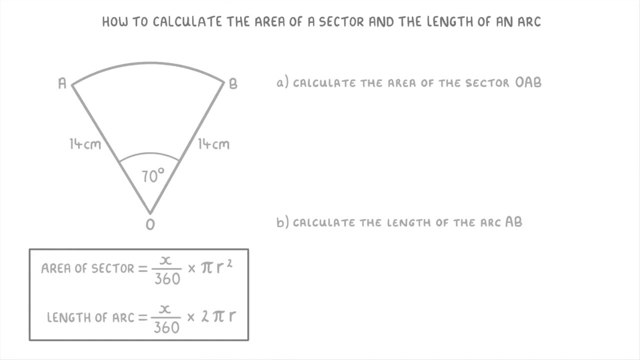 millimeters. Before we finish, let's have a go at this question here using the two equations from the start of the video, And remember that the x just means this angle inside the sector. Also, don't worry that here we're only given the sector, not the entire circle. Sometimes they'll 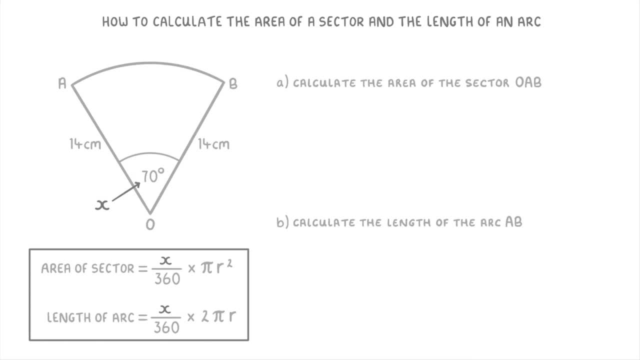 just give you this sort of shape and they'll tell you that it's part of a circle, or they'll give you the radius. And if they give you the radius, you know it must have come from a circle. So for part A, it's asking us to find the area of the sector OAB, And OAB is just a way of. 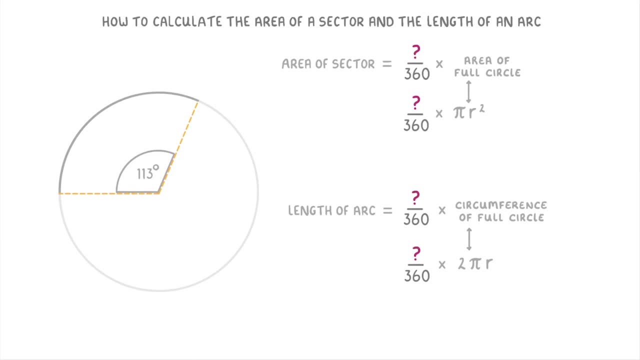 360 degrees in a circle in total, and then you just place whatever angle your sector is as the numerator. So in this case, because the angle of the sector is 113 degrees, our fraction would be 113 over 360, or in other words, our sector is 113 360ths of the circle. 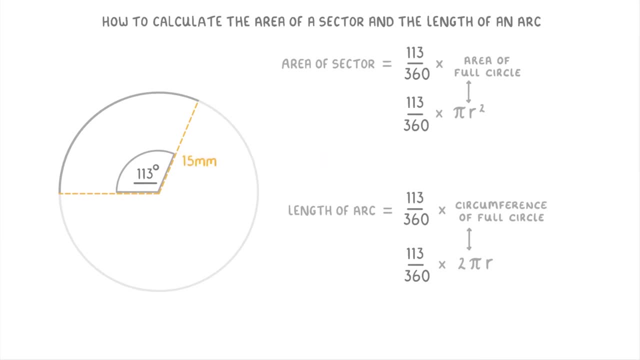 So if the radius this time was 15 millimetres, then to find its area we'd do 113 over 360 times pi times 15 squared, which would be 222 square millimetres. And to find the length of the arc we'd do 113 over 360 times 2 times pi times 15, which is 29.6 millimetres. 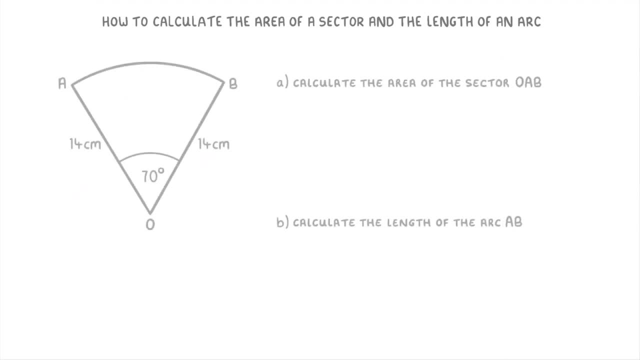 Before we finish, let's have a go at this question here using the two equations from the start of the video, And remember that the x just means this angle inside the sector. Also, don't worry that here we're only given the sector, not the entire circle. Sometimes 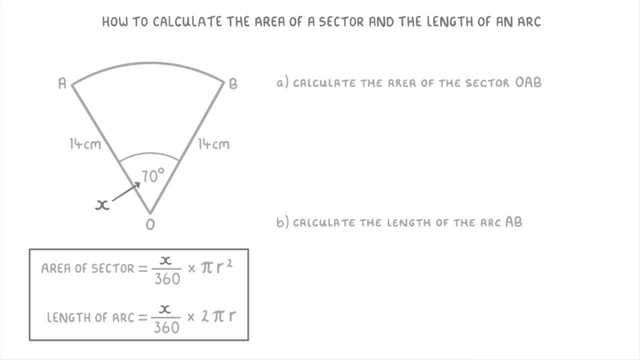 they'll just give you this sort of shape and they'll tell you that it's part of a circle, or they'll give you the radius. and if they give you the radius, you know it must have come from a circle. So for part it's the same thing as before. If you've got the radius, you know it must. 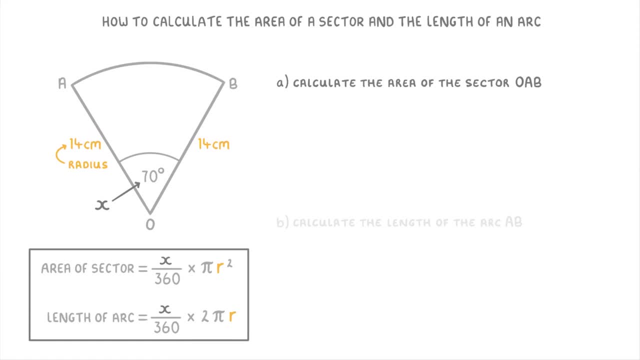 have come from a circle, So for part it's the same thing as before. If you've got the radius, you know it must have come from a circle. But notice that it's asking us to find the area of the sector and is just a way of describing the sector. on, 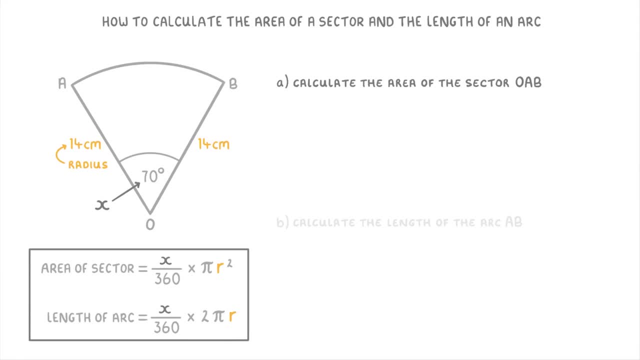 the left, because O, A and B are points around the shape. So we're going to use our equation. area of sector equals x over 360 times pi, r squared, which, if we sub in the 70 degrees and the 14, will be 70 over 360 times pi times 14. 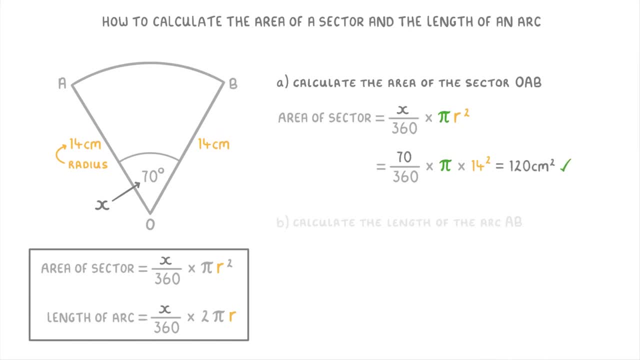 us 120 square centimetres. Then for the length of the arc AB, so just the arc in between A and B, we do x over 360 times 2 pi r, which will be 70 over 360 times 2 times pi times.